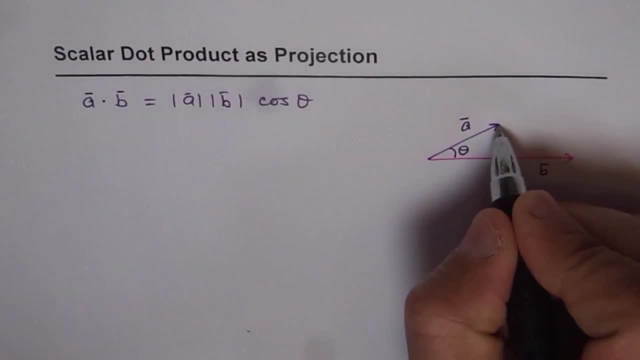 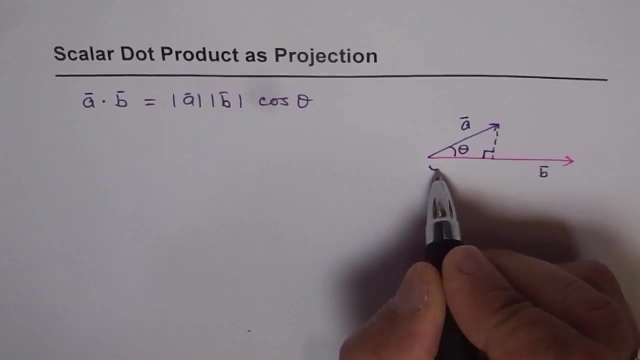 b. So this is the projection of vector a on b. Projection is like this: So this is the projection of vector a on b. So how much is this length? That is the right triangle, correct? And this is the hypotenuse. This becomes adjacent side of the hypotenuse, correct? So let's say this is o and. 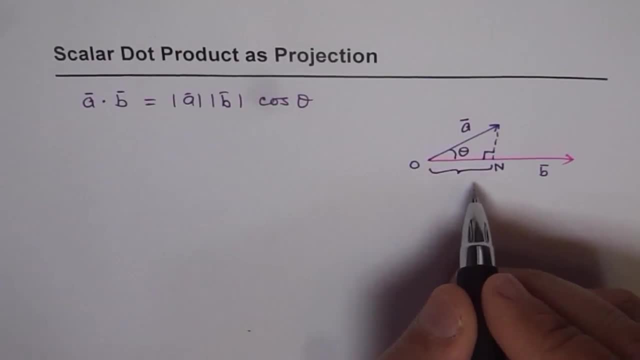 this part is n, Then this length will be how much? So we can say o n over magnitude of b times magnitude of a is equals to cos of theta, right, And therefore we can say o n is equals to magnitude of a. Let's write magnitude, So magnitude of a times cos of theta. That is this length, o n So. 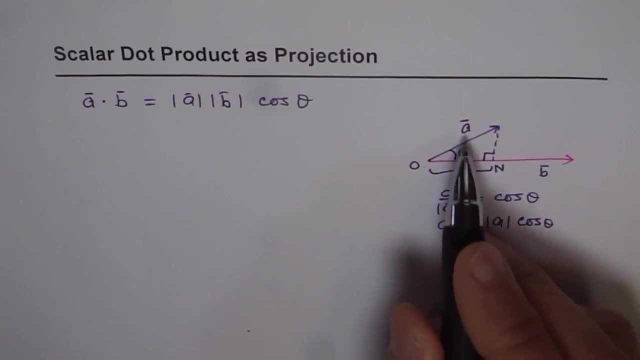 basically, o? n is projection of a on b, right, So we can write what is o n? So we write o n is projection. let me write on B This kind of symbol, right? It is also a symbol normally used for projection and we'll. 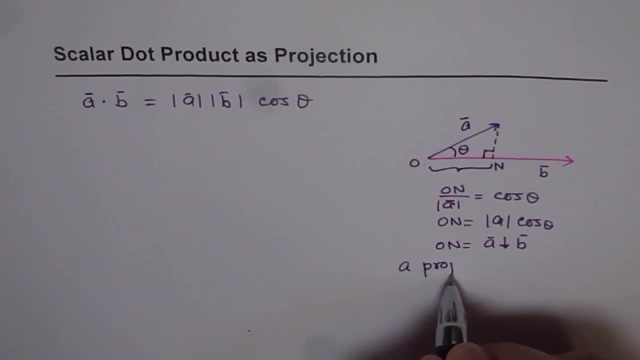 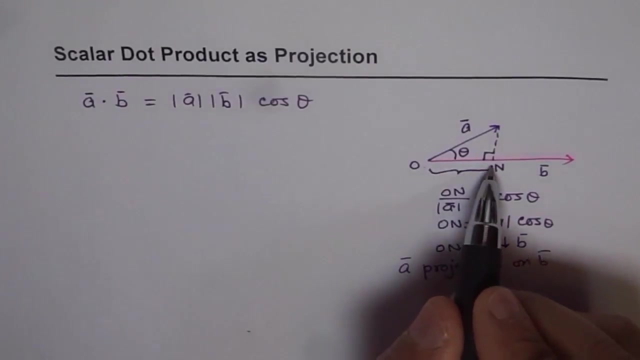 read this as A projection on B, right. So vector A projection on B will be ON, correct. Or you can say: the component of vector A along OB is ON, correct, So that becomes ON. So we see that ON is actually equals to absolute A times cos theta right. Now, if we rearrange this formula, 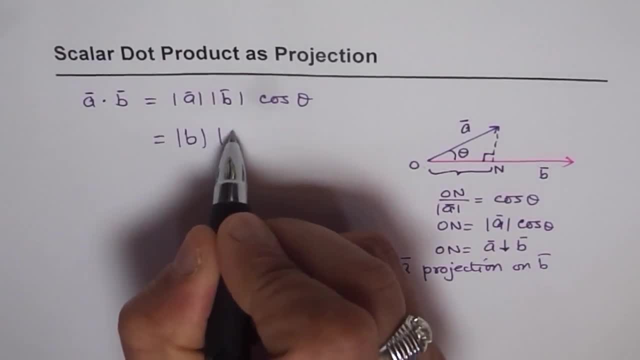 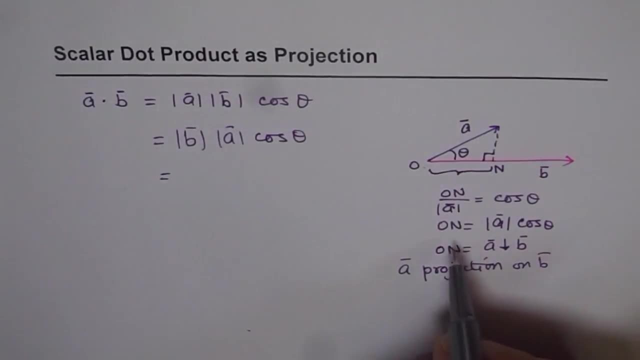 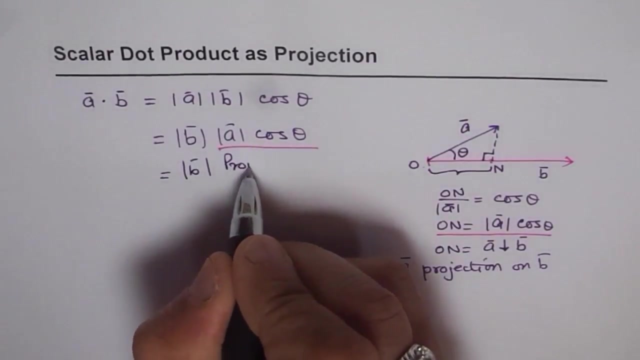 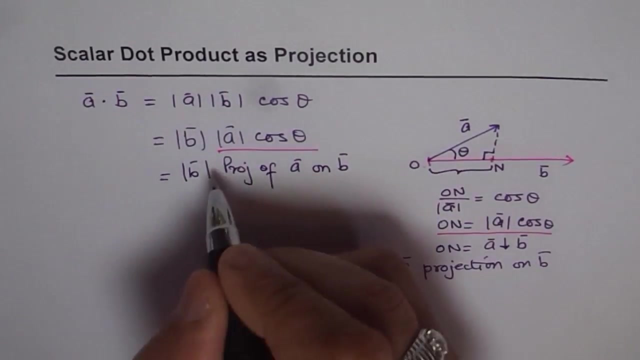 we get what We get: B times A cos theta right Now here. if you compare the two, that means what we're trying to say here is A cos theta and ON. You see this part. So that means magnitude of B. whatever this vector is times projection of A on B, do you see? So that is how you can relate. 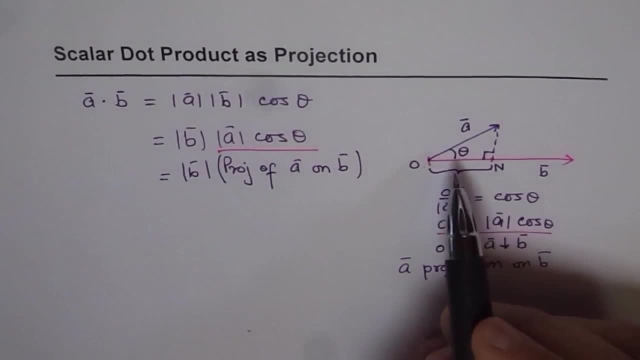 the dot product. So dot product basically the component of A along B, or projection of A along B times the magnitude of B right. And from this property we can also get all other relations, That is if my angle theta increases. 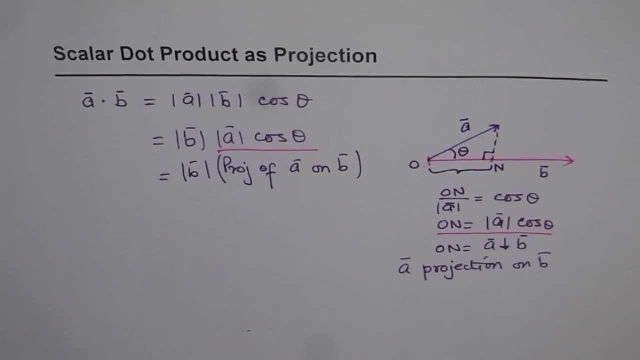 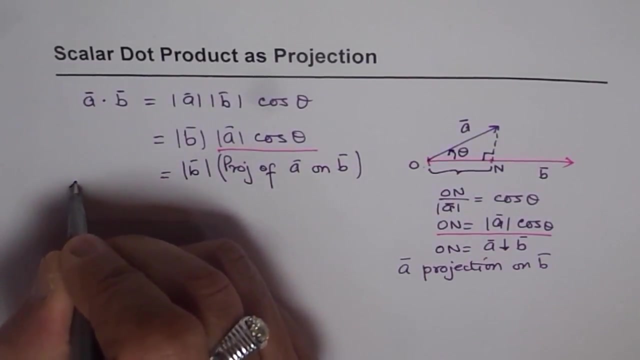 then what happens? right? So let's look into those conditions. Now, if let's say this is my vector B, Now let me draw it here, vector B, And now what I'm trying to do is I'm trying to increase this angle, theta, and if the angle becomes vertical, right In that. 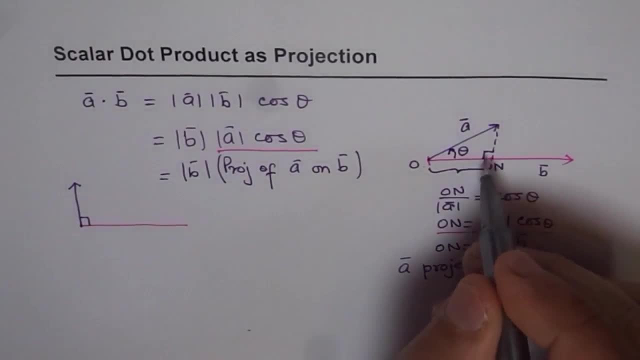 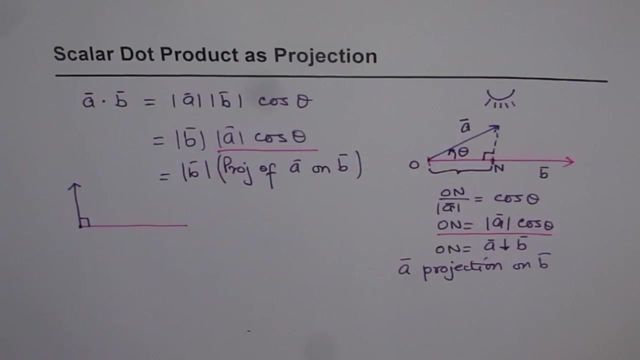 case, let's say this is my angle vertical, then the projection projection is like a shadow. If I have a sun here and then where will the shadow fall, It will show me the projection there. Do you see that? In this case, what is my projection of A on B? 0, right, So? 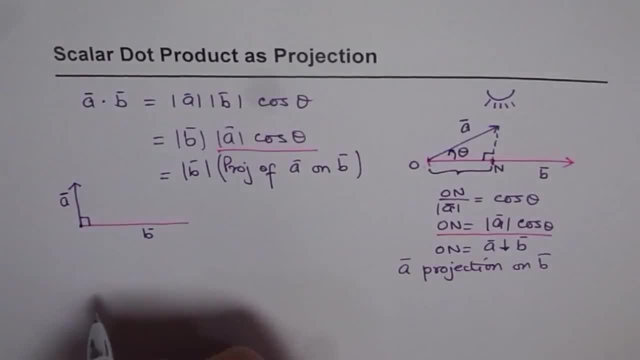 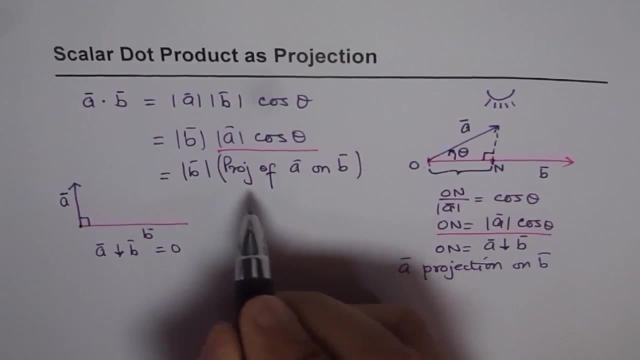 this is my vector A and this is my vector B. Now, in this particular case, the projection of A on B is 0, right, So this part is 0. So that means A dot B equals to magnitude of B, whatever it is. 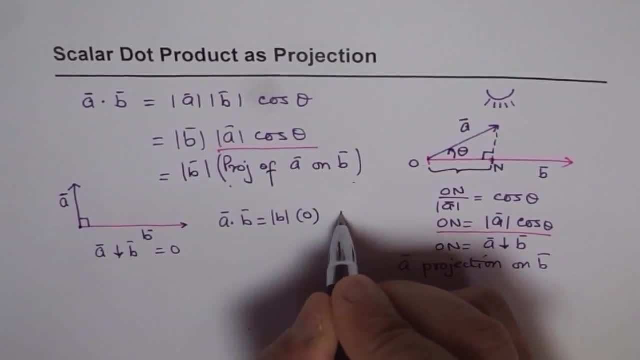 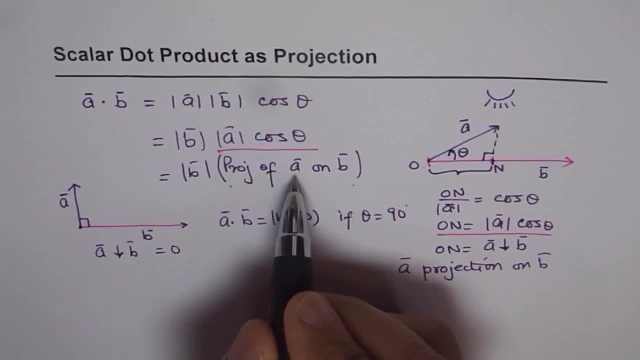 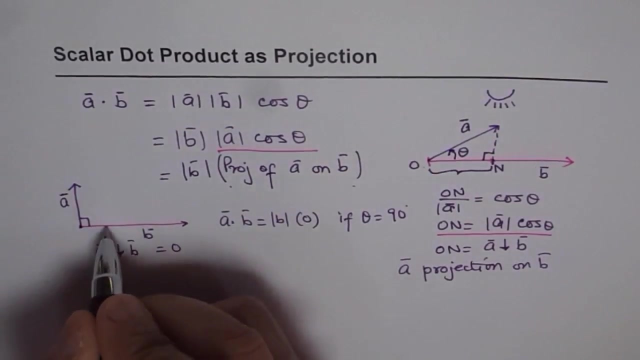 right Magnitude of B times 0, if theta equals to 90 degrees, which you get from the formula. also, since the projection of A on B is 0, correct, And you'll also see if I move, if I increase theta, as I increased theta. 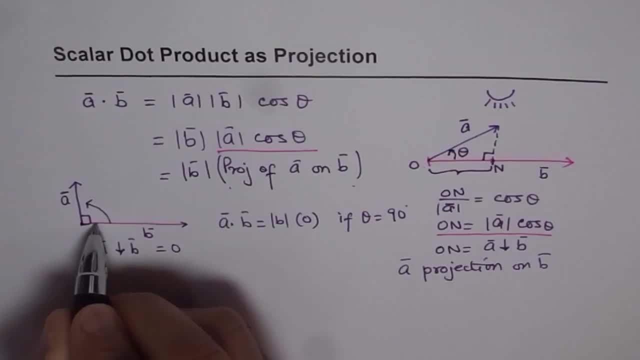 from zero. So when it is at zero, let's say this is my initial position of A, let us say right At that time, the projection is same as the magnitude of A right. As I increase my theta, the projection decreases, correct? 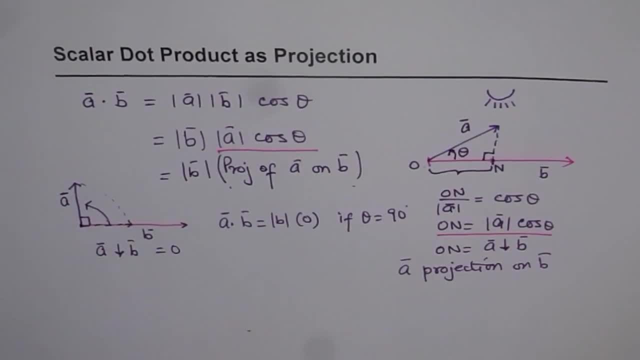 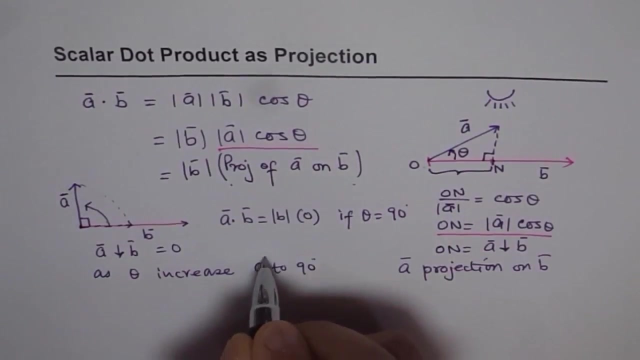 And it becomes ultimately zero at this stage, correct? So the product which we are calling dot product or scalar product will decrease in magnitude. So as theta increases, so we see that as angle theta increases right from zero to 90 degrees, what happens to the dot product? 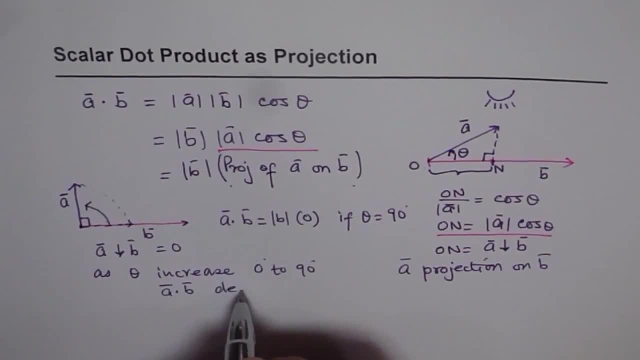 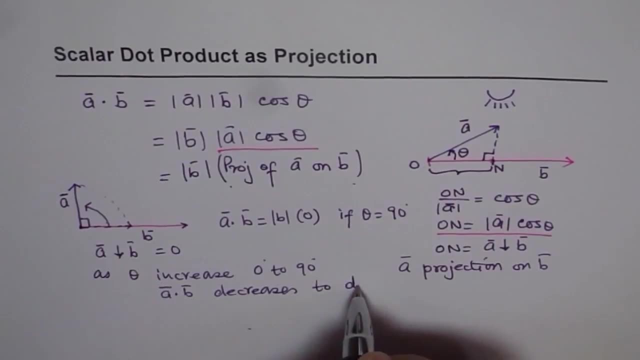 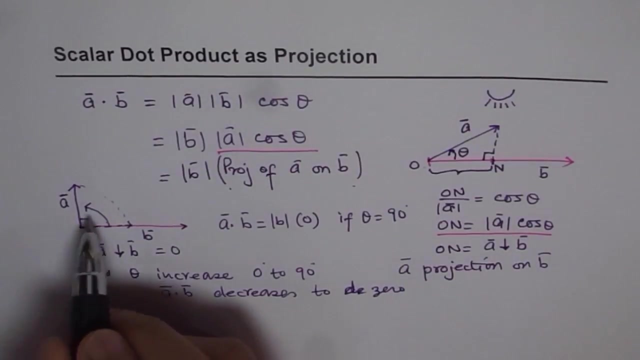 A dot B decreases right from maximum to zero. Do you see that A dot B decreases to zero when theta is 90. From maximum to zero. Do you see that? So that is how it changes, right? When we do it in the other direction, then cosine of theta becomes negative, since cosine theta is negative for angle more than 90 degrees, right. 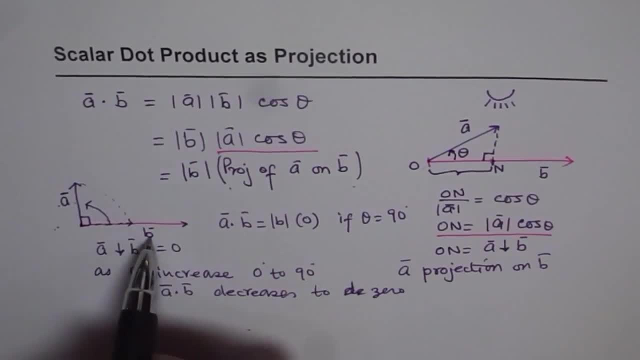 The other thing is that the direction of projection is reversed from B And therefore we have a negative value, kind of right. So this is our reference point, zero. So it is like a reference number And the magnitude in this direction is taken as negative. 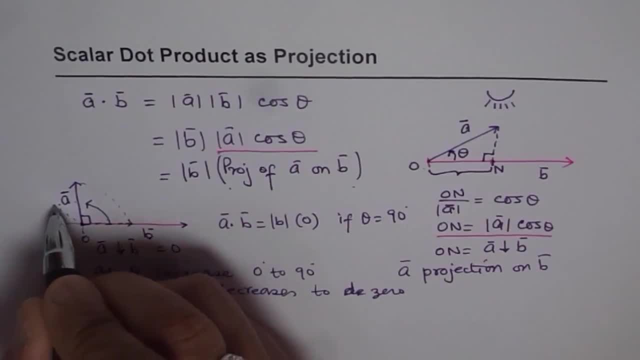 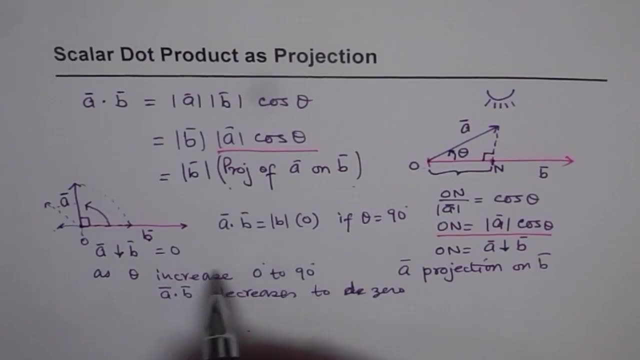 And therefore the projection. as we increase this again, then theta. as theta increases from 90 onwards, we get more negative values. Effectively, it decreases right from zero to negative. So it keeps on decreasing from zero to 180 degrees. 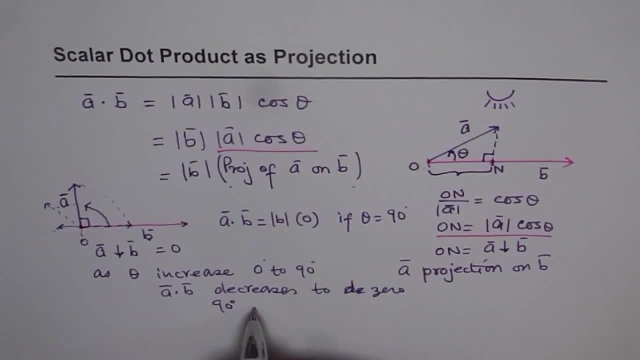 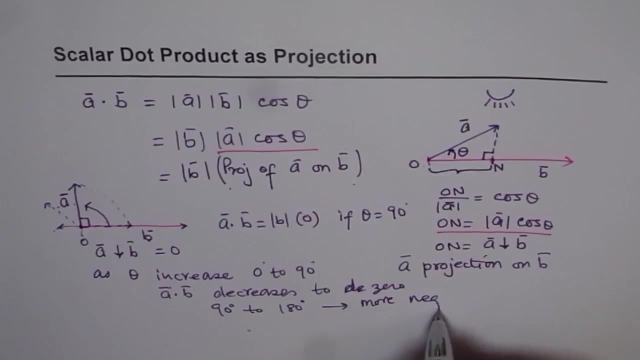 As we move further- now, as we move from 90 degrees to 180 degrees- then what happens? It becomes more negative. Negative because it points towards negative x direction. It becomes more and more negative. So that is how it can be interpreted. 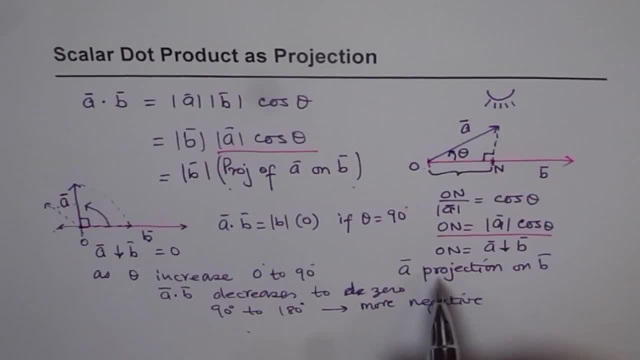 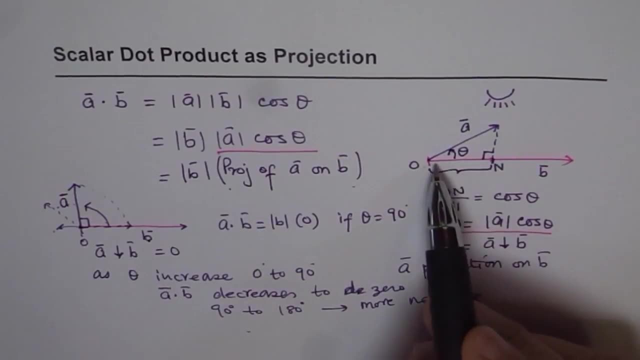 But effectively, if you see the magnitude-wise, the component of A which is on B, or the projection of A on B, really gets multiplied by the magnitude. So what is the magnitude of B when we are finding a dot product right? 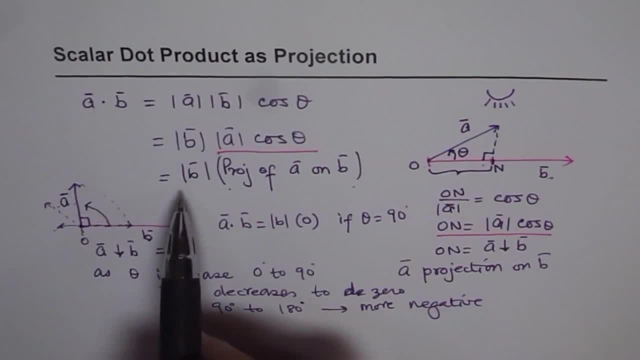 So dot product can be seen in short as A dot. B equals to magnitude of B times projection of A on B right. So that is the relation between the two And from here if you want to find what is projection of A on B, 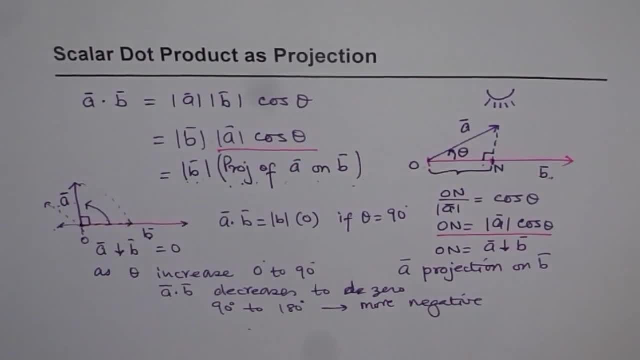 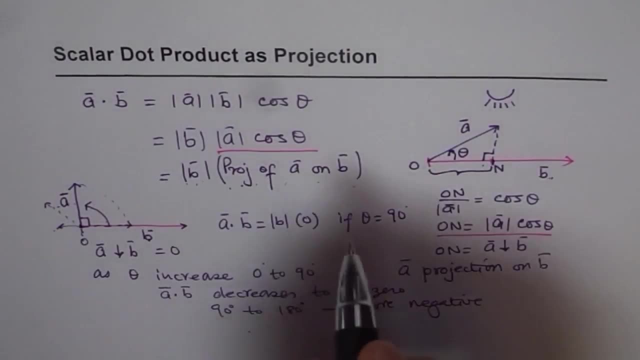 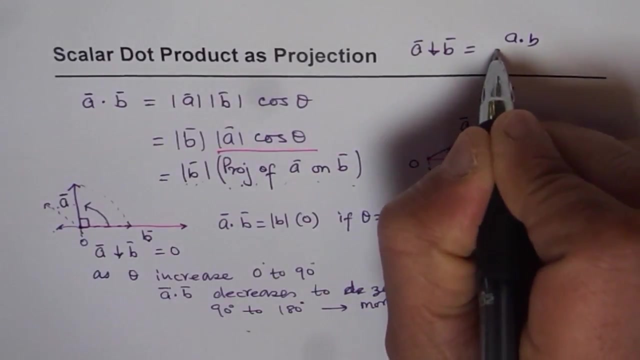 it is A dot B divided by magnitude of B, correct? So that is what we can summarize here, That projection of A on B. so we say projection of A on B is actually equals to A dot B divided by magnitude of B, correct? 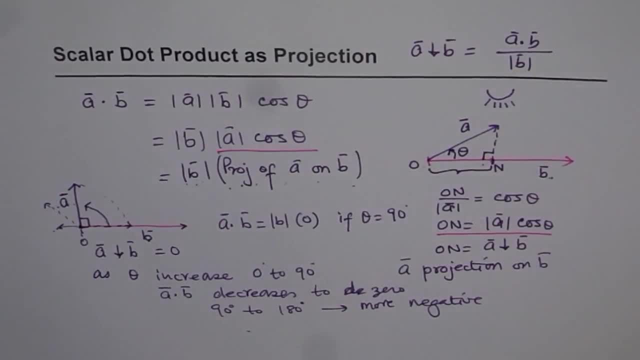 Such an important formula we can get from this simple concept. I hope you appreciate it. And this projection which we are talking about is scalar projection, mind it right, Since the dot product is giving us scalar quantity. But if you want to make it,